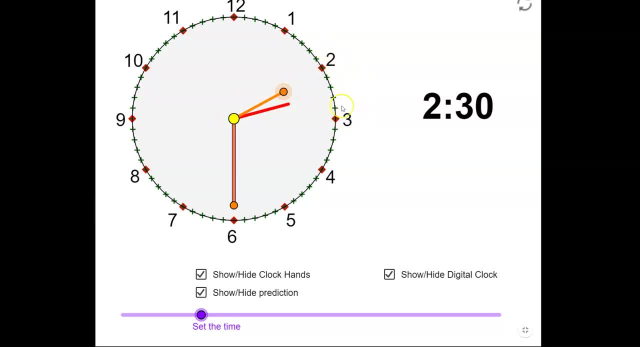 in a specific point within the two and three. So that's something I would love to see changed about this. And I do, again, really love how you can hide and show the hands for the prediction for the clock, for the digital clock, Because when you're teaching it and you're beginning to 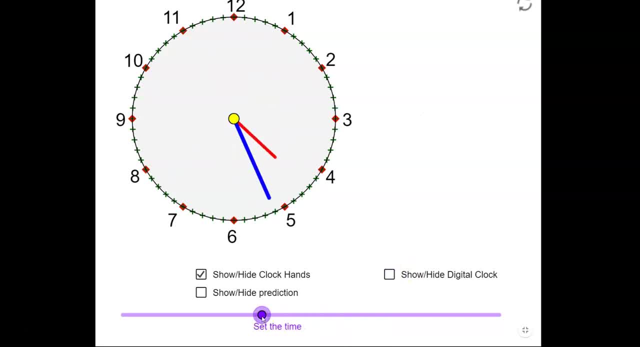 quiz students a little bit. you want to hide the digital clock and you want to ask them: what time is this? They might say five because the hour hand is super close to five, or they might say four because it's in between the two. But you go ahead and ask them. they make their. 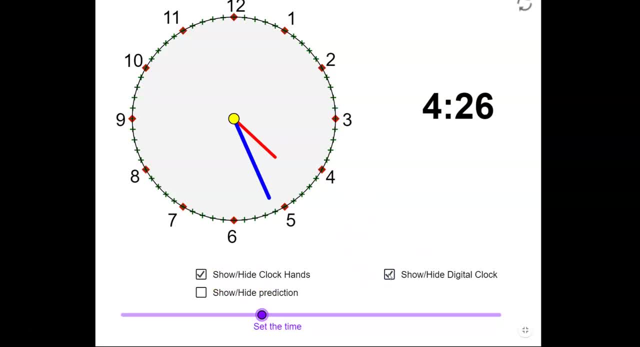 prediction, Then you show it and you can explain why the time is what the time is with the show and hide digital clock. I do wish you can make a specific or type in a specific time within the digital clock because, as you saw, I did struggle to get to a specific number. but that can be improved. 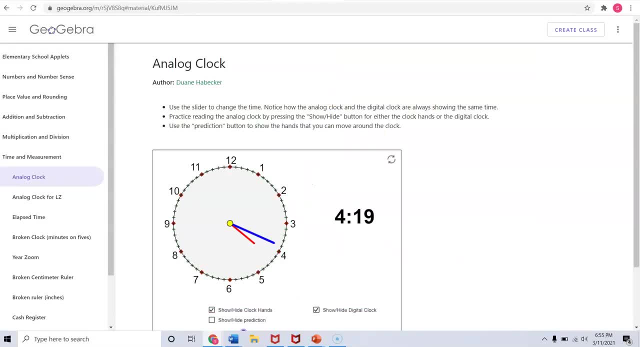 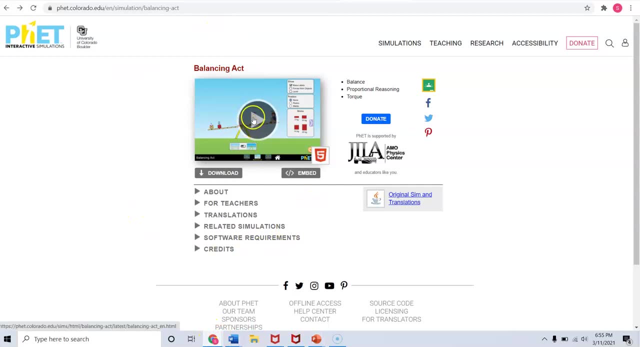 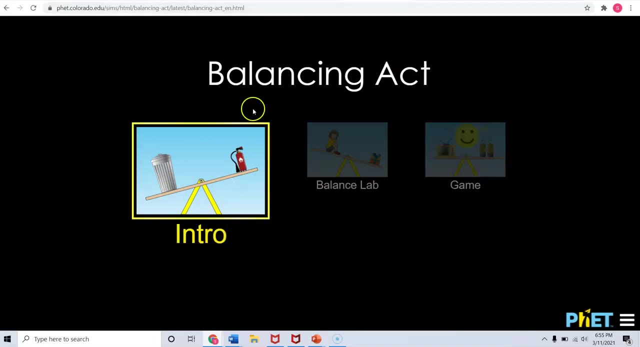 within time. The second one I'm going to show you is FET simulations. Again, multiple tools, multiple tools, Multiple grades. but we're going to focus on the balancing act. So the balancing act, or just most of the FET simulations in general, have an intro, a lab. 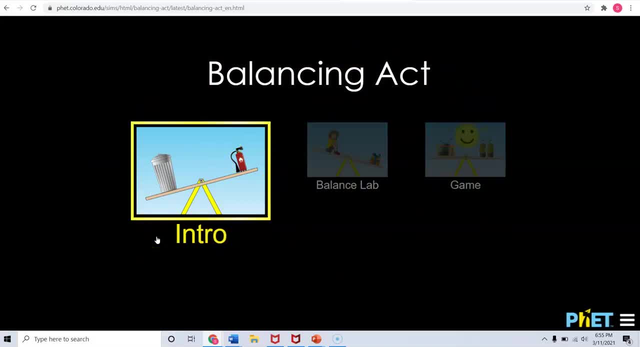 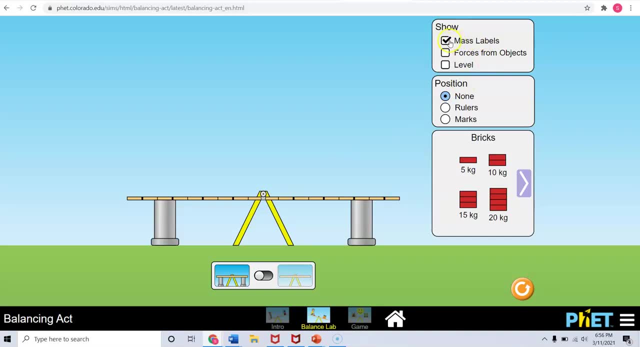 and some have games. The intro is just to play around to get the feel for how to use it, But then you're probably going to most likely use the lab. You can go ahead and show the mass labels or not. So if I drag this mass on, it's not going to tell you that's five. 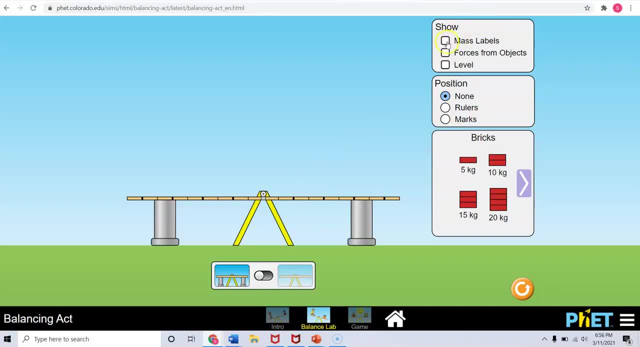 That's something that a teacher would decide if they want to use or don't use. But you can also show the force that the object's going, if it's going up or down, and you can show if it's level. You can also measure how far from the center it is and you can also put marks so you can see if. 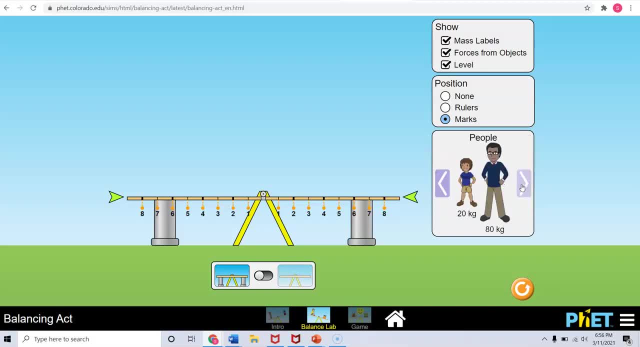 something's going. There's different weights that they provide people, and then they also have mystery objects. My one thing is that you can never unveil the exact weight of an object without measuring it through. Now I already went ahead and realized that these are the same weights.